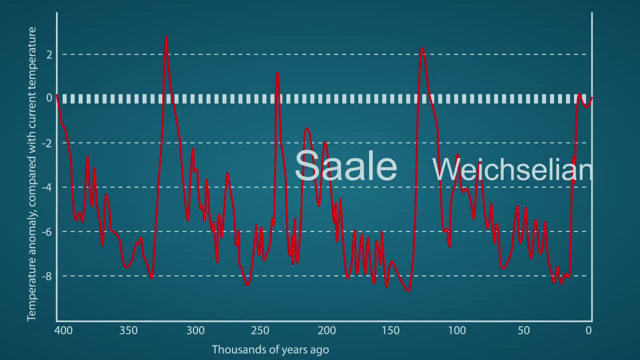 the Weichselian glaciation. Both periods have had a lot of influence on the formation of the landscape in northern Europek, in Northern Europe and on southern Europe. however, you can check The Sala glaciation. the second last ice age, occurred about 238,000 years ago to 126,000 years ago. 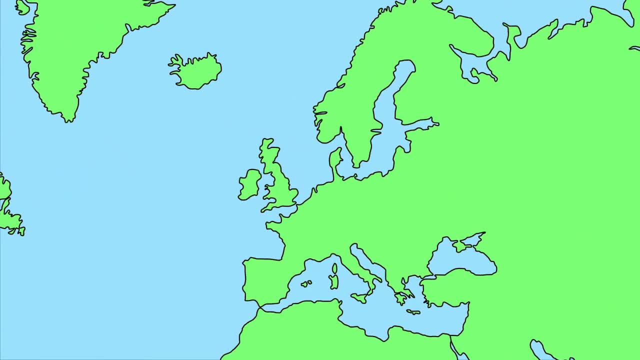 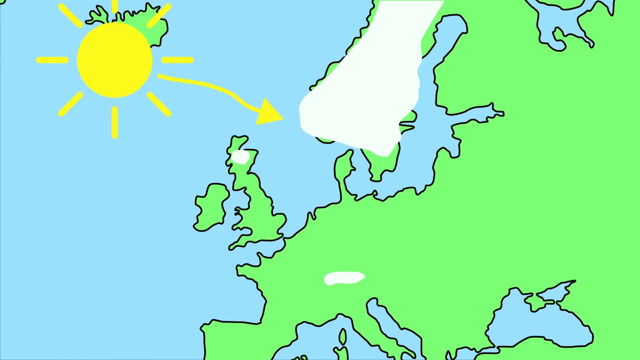 Because it was very cold, on average about 6 to 8 degrees cooler than today. ice caps formed in mountainous areas because it is colder there due to the altitude. Because this huge pack of snow and ice also reflected a lot of sunlight, it could remain cold on Earth. 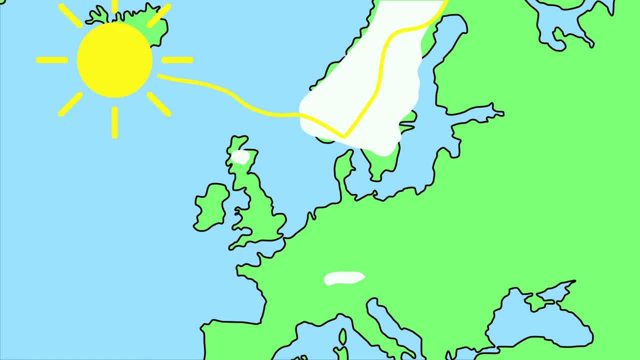 There was a lot of ice on the continent, so that the global sea level was tens of meters lower and shallow seas became dry, such as the North Sea. In Scandinavia, too, more and more ice formed in the highlands, which did not melt due to the cold climate, but slowly moved to the rest of Europe and formed the landscape. 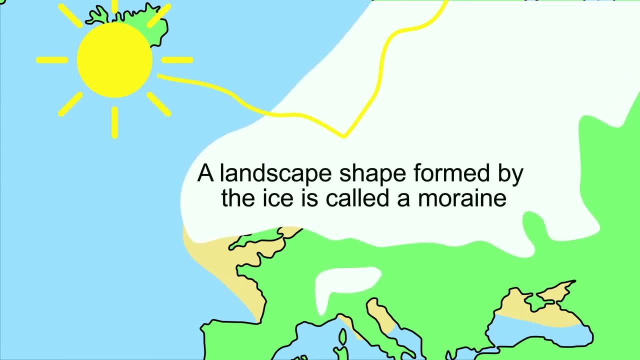 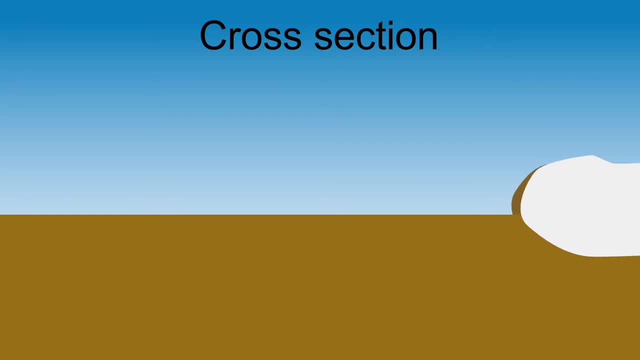 A landscape shape formed by the ice is called a moraine. Some material is deposited under the ice. This type of soil consists of an unsorted mixture of clay, sand and boulders and is called boulder clay. This is called boulder clay. 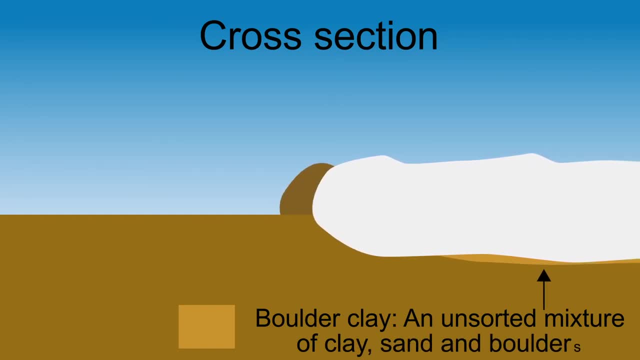 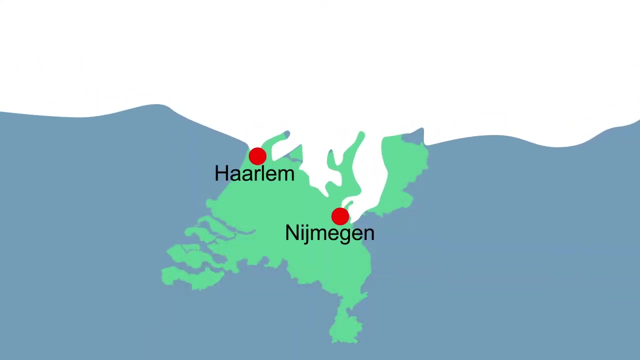 The moving ice has also pushed away parts of the soil. Debris that is carried along by a glacier is accumulated, forming moraines. These hills are called push moraines. The land ice from Scandinavia slowly moved to the Netherlands approximately to the Haarlem-Nijmegen line, pushing sediment upwards and creating push moraines at the end of the land ice. 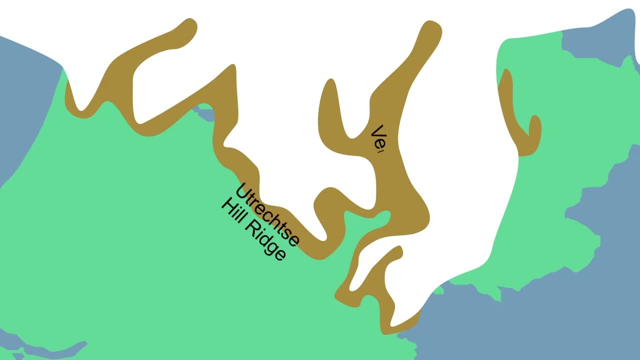 These push moraines are now known as the Utrecht Hill Ridge, the Veluwe and Saaland Hill Ridge National Park. When the bottom was scraped away, a hollow is left behind by the ice mass. These deep parts are called tongue basins. 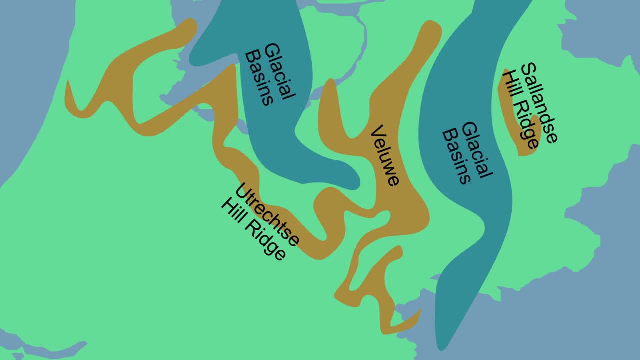 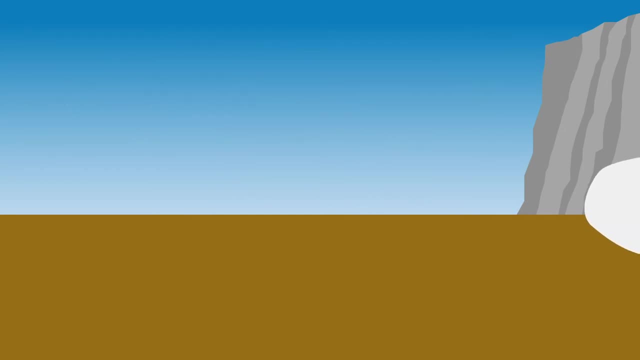 Because they are formed by ice, they are also called glacial basins. There are a lot of tongue basins. When stones fall onto the surface of glaciers, they are carried along by the ice and they are called glacial erratics. 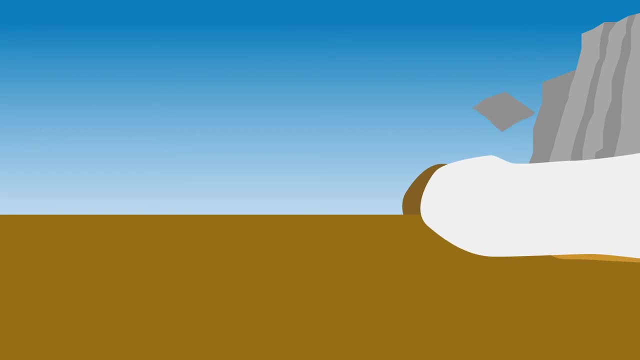 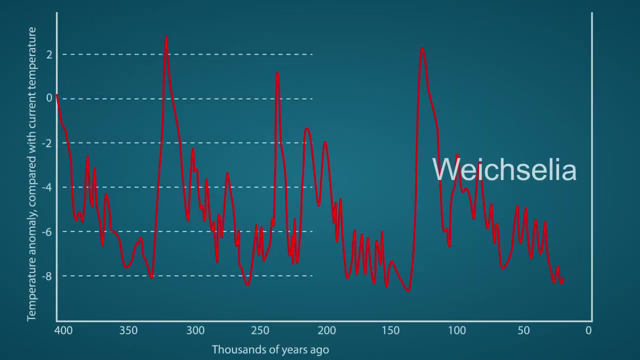 When the ice melted, the stones remained in the landscape, as in the Drenthe region. Because the land ice spread to the Haarlem-Nijmegen line. there are no boulders south of that line, The Weikselian. the last ice age lasted from 116,000 years ago to 12,000 years ago.